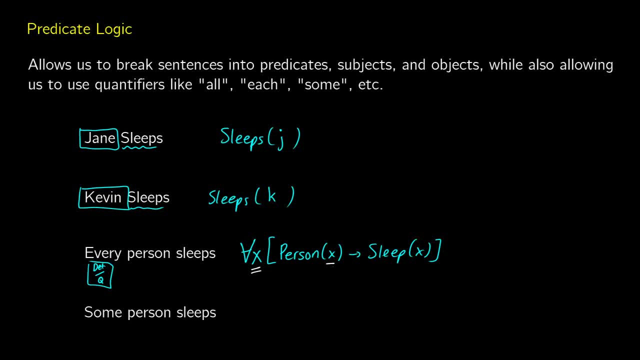 our universe x. we're going to take a look at every x And for every x that is a person, x is going to sleep. Similarly, if we have some person sleeps, we can use a new operator called the existential operator. We can say there is some x out there, such that x is a person and x sleeps. 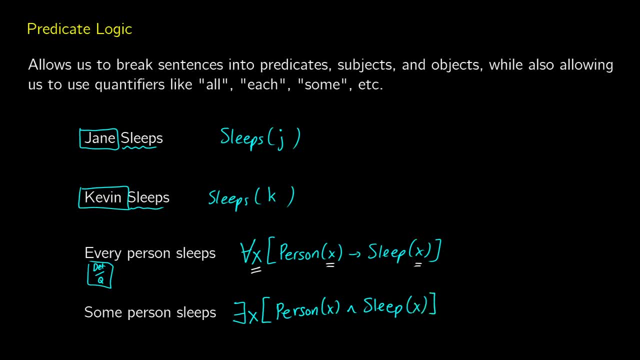 So if you're not quite sure how to do the translations for these, of course we're going to cover them a little bit more slowly after, But just to show you the power of what predicated logic can and can't, Because in our old system we just have to say j, k, e and s, and that's not going to get. 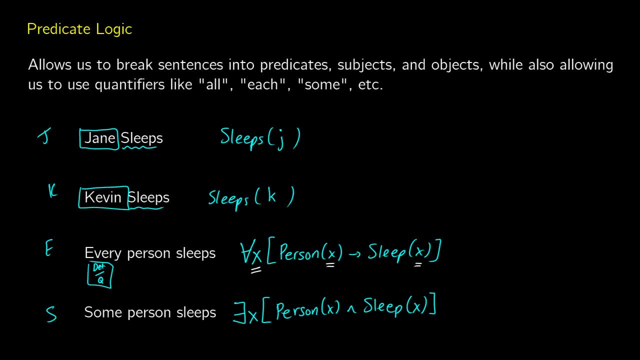 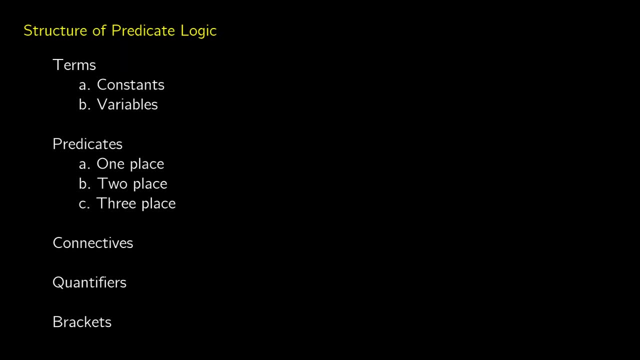 us the details of what's similar across all of these things and allow us to evaluate the truth of these more complex sentences. So here's our structure of predicate logic. We start with these things called terms, and these are basically everything inside of our brackets. So what you? 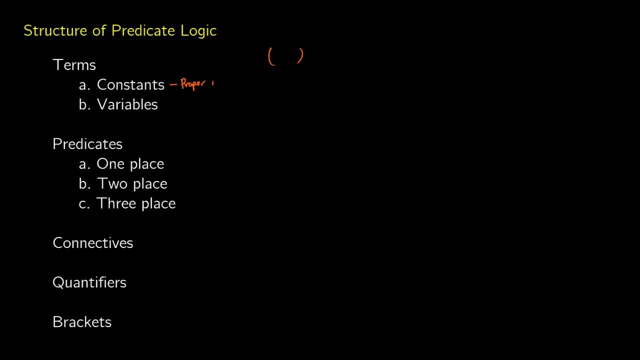 can think of with constants is you can think of them as proper names. So for proper names, typically we use lower case letters and we start at the beginning of the alphabet, and this usually goes all the way up to about t For variables. you can think of these as pronouns. So we usually start with lower case x, y, z. 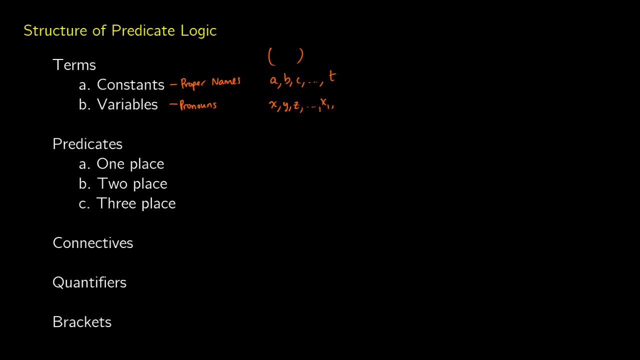 Sometimes we give them subscripts like x1, x2, and so on and so forth. Sometimes we give them subscripts like x1, x2, and so on and so forth, so on, just in case we need more letters. but if you have something like sleeps x, well, this is what. 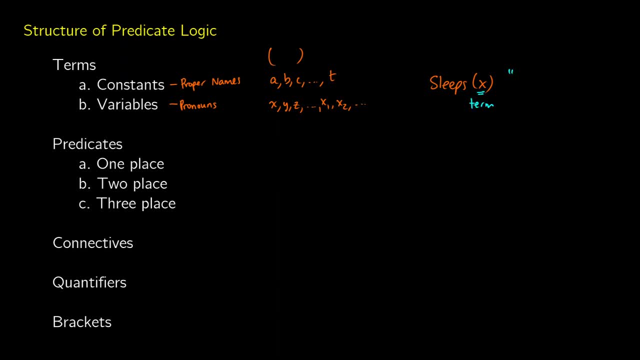 we're talking about, when we talk about a term, and you could think of this sentence as being something like he sleeps, we don't know who he is. that's why it's just a variable there. we need something in the real world to tell us who he is. but this is where you would put your subjects, your direct. 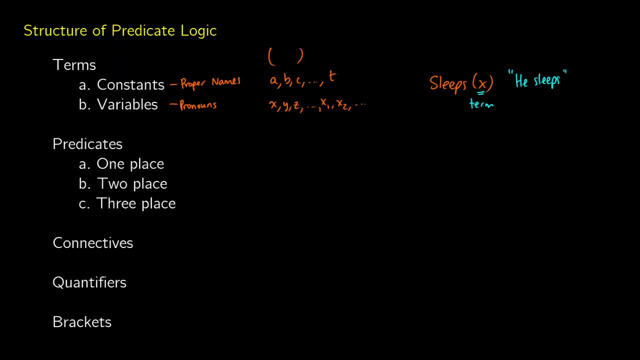 objects, your indirect objects, and so on. now we have predicates, so we usually think of these just as verbs, but they can be nouns and adjectives too. so, for example, we might have one place predicates and these would be your intransitive verbs, these would be your common nouns and these 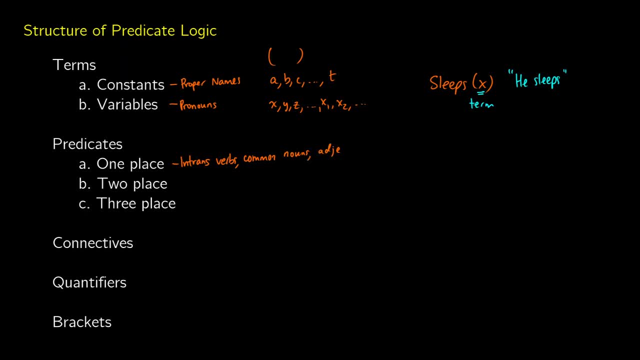 would also be your adjectives, so you might think of something like dog x to mean that x is a dog, or maybe something like happy x to mean that x is happy, or even something like we saw before with sleeps. we might have another verb that's intransitive. 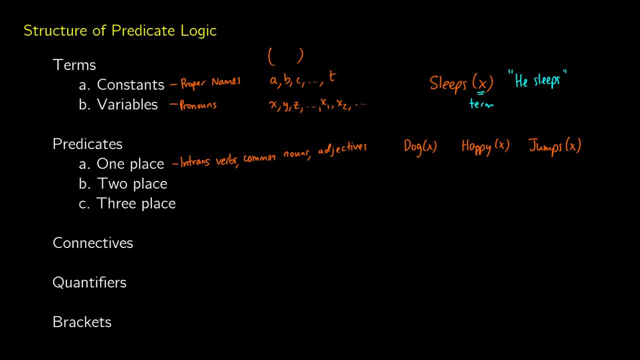 like jumps x, to mean that x jumps. with two place predicates. we usually think of these as our transitive verbs or our prepositions, since prepositions usually relate two things together. so it might be that someone- let's use a different example here, we'll see this one a lot today- likes so, x, likes y. so we can put our subject. 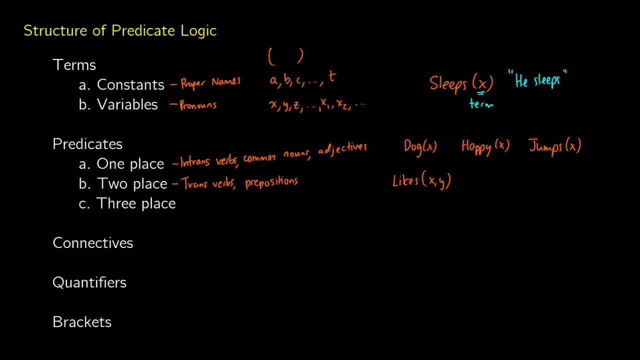 x and our direct object into that predicate, and those would be two different terms. or if one place is inside of another, like if we say that vancouver is in canada, then we would have x is in y, so we would do in and then x and y as are two terms there. now three place predicates would be: 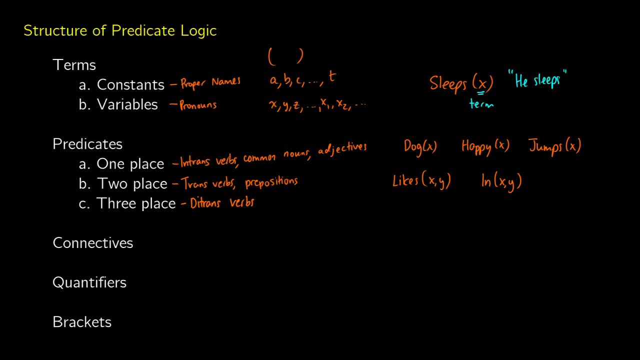 our di-transitive verbs. so this would be something like gives. if you have gives, you can have a sentence like x gives y to z. so we can put in three different terms there: x, y and z. we'll call x, y and z our terms or our arguments, and this would give you a sentence like x gives y to z. 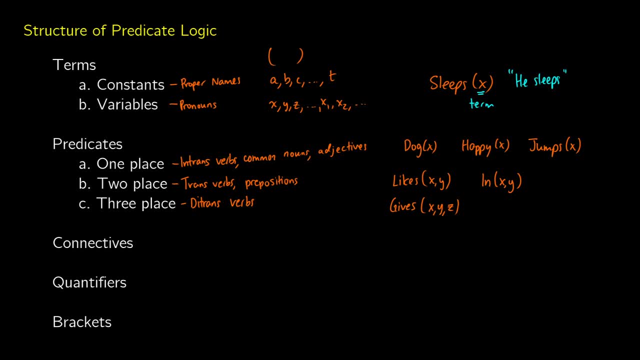 or x gives y, z depends on how you phrase it. now, as far as connectives go, we're going to have all of the standard ones that we had in propositional logic, so you should for all of these ones. so we're not adding anything new. we may talk about the identity operator a little bit later. 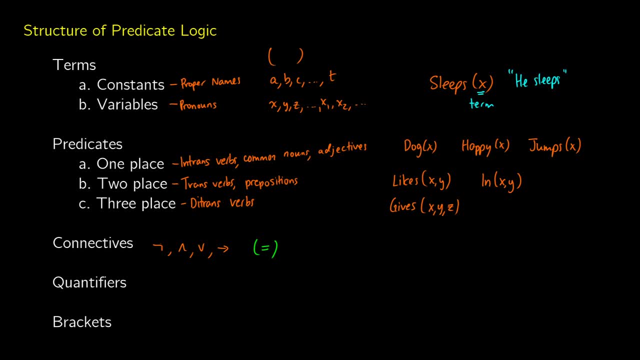 that is included in predicate logic, but we'll forego that for now. so we do have an identity operator for quantifiers. we have two new ones. so this is the upside down, a, which means for all, and the backwards e, which means exists or sum. and finally we're going to have our brackets, so we 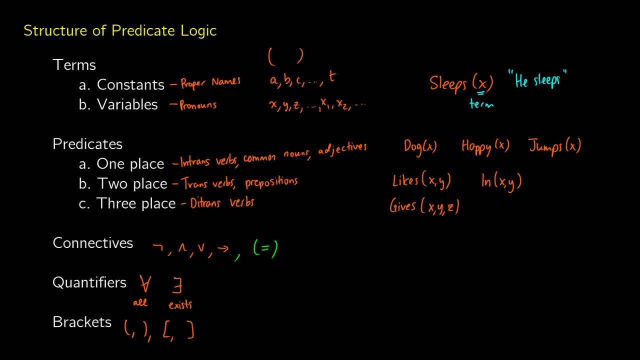 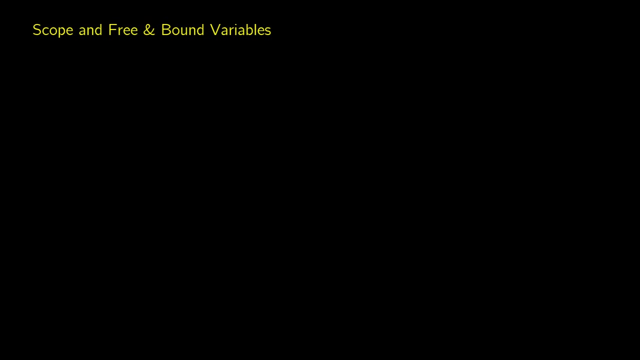 have our parentheses, and we'll also introduce square brackets just to make some things a little bit easier to parse. so these are all the tools that we have at our disposal, and let's see what we can do with them. now, one of the things you'll come across with predicate logic is this thing called scope. 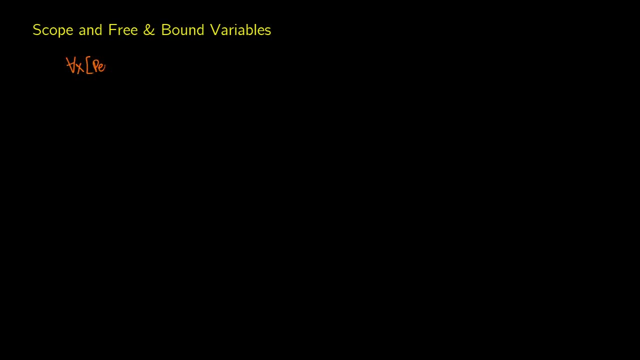 so imagine if i had these two different translations for all x and then i put person x in brackets and i say happy x outside of the brackets, and then i have something that says for all x, person x and happy x. so each of these have slightly different translations and that's due to this thing. 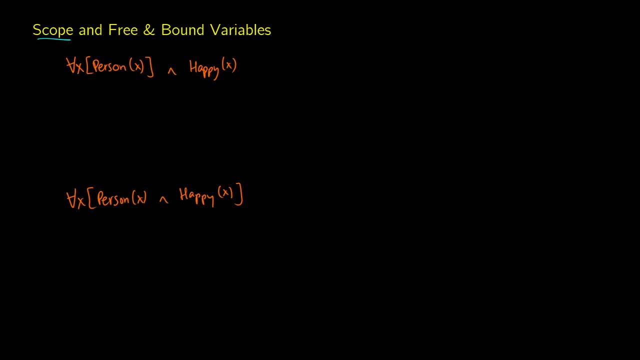 that's called scope. so whenever we have a quantifier, like for all x here, this has a scope, and the scope starts from the bracket that initializes it to the bracket that ends it. so we could say: the scope as for for all x here is just person x, and what this means is basically. all people, all people. so the all-ness is only Religion, which means all persons. equal for x is equal for all. x for all. x means for all people거든onull: patient, person, percent and score and bosses range for political border analysts, Jr. Now, if this is a lot of people, we need to make this something lessvl. 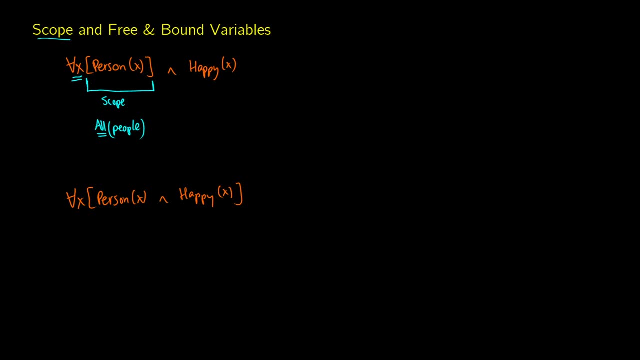 only being too restricted to the fact that we have people there. So if we were to translate this into English, we'd say that something like every x is a person. So this is one bit of information And x is happy. But the thing about this is is that these two x's are not the same. 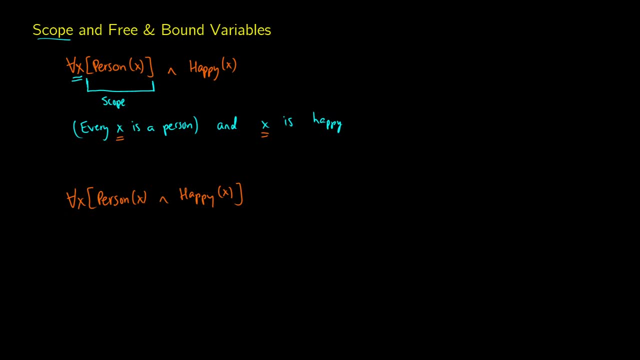 x's because the scope of for all x is only covering person x and not happy x. So we can think of every x is a person as being something that is bound, because whatever is in our scope is going to be bound by that quantifier, While we can think of this other x as being what's called 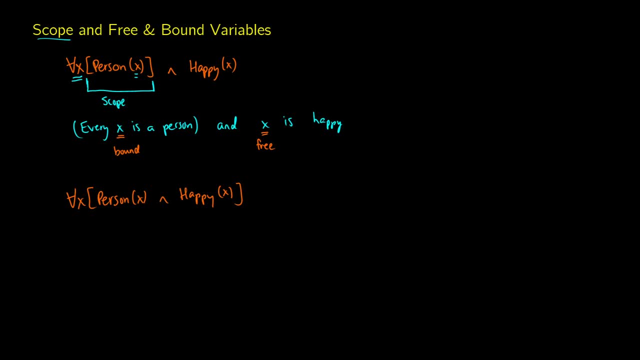 free because it's not in the scope of our quantifier. So if we want to think of the sentence with a better translation, you would say something like everyone is a person. that would say, for all, x person, x, And because x in this case is a free. 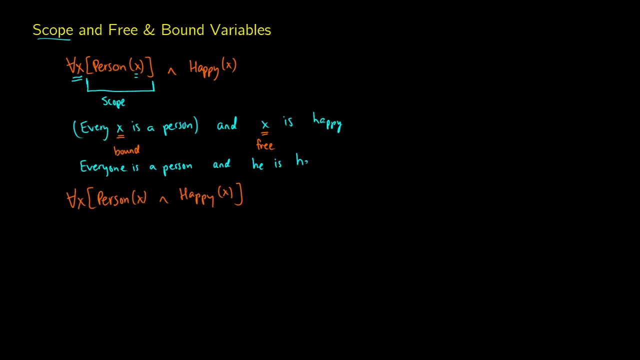 variable. we think of it as a pronoun. So everyone is a person and he is happy. So if we compare this to our second one, for all x bracket, person x and happy x bracket, what this is doing is, this is taking both of these predicates under its scopes. So we can say: 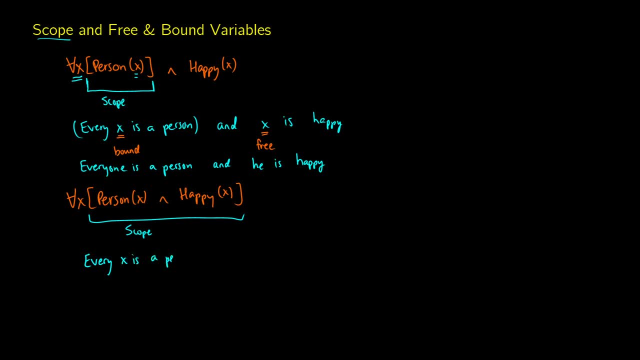 here, every x is a person, And this every will also go over to the x under happy, though, and every x is happy. So if we think of this more in an English translation, we could say something like every everyone is a happy person. 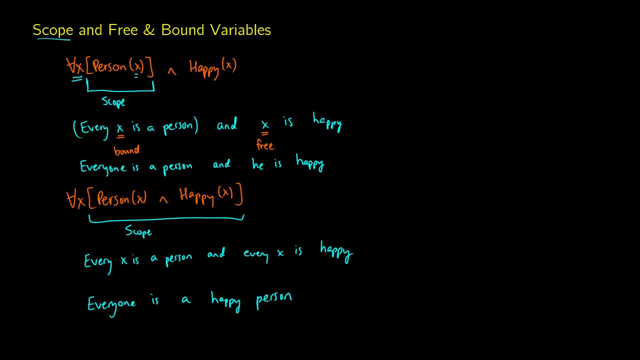 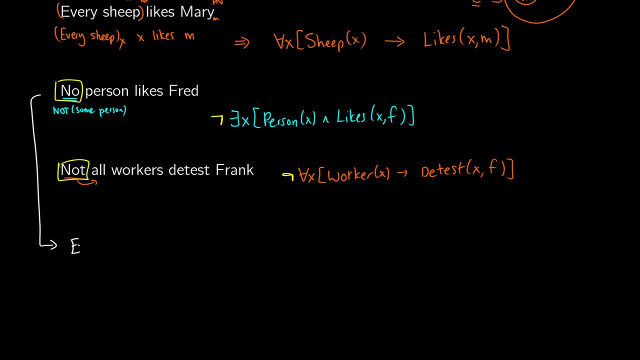 for all x, when you think about for all x. when you think about for all x, when you think, If no person likes Fred, that's the same thing as saying that every person does not like Fred. So if we do it this way, we can translate it in a slightly different way. 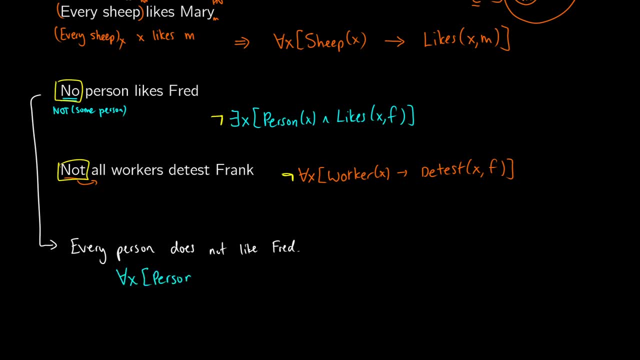 We can say: for all x if x is a person. this is just our all people translation. But now we have: does not like Fred. So what we can do is instead we can negate our predicate here. So for all x if x is a person, then it is not the case that x likes Fred. 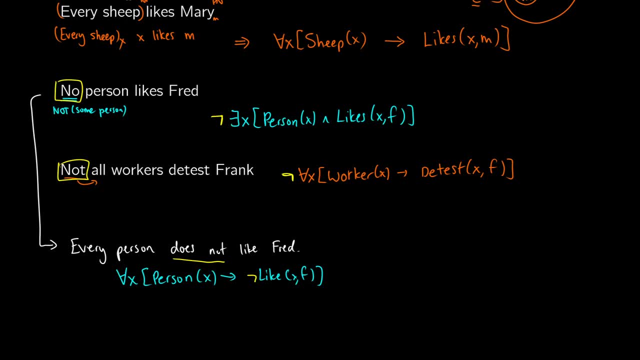 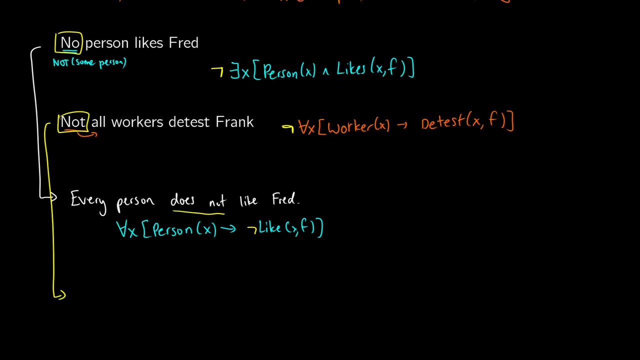 So this would be an example of a paraphrase of no person likes Fred. Now, if we were to do a paraphrase of not all workers detest Frank, well, if not all workers detest Frank, what does that mean? That means that there's some person out there and they do not detest Frank. 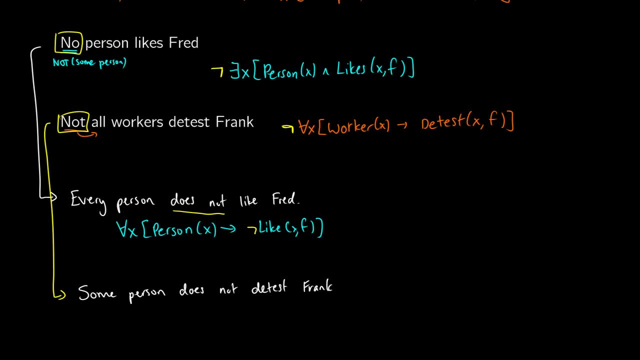 So some person does not detest Frank, Then when we do our translation here we're basically saying some person. so there exists an x such that x is a person and we use the and with the existential does not is going to negate our predicate. 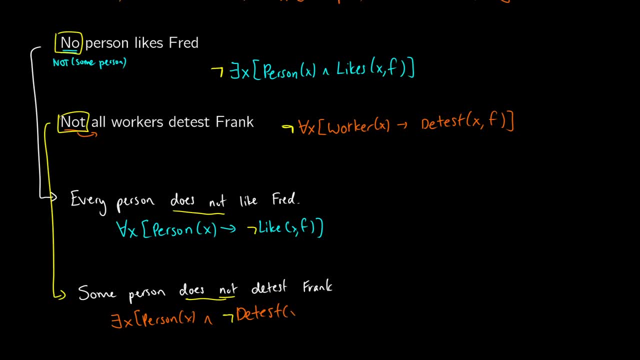 There. this is, this is going to be. the rest is normal to test x and Frank. So with the cases of no one, not all, there are two different ways of translating these sentences. Either the negation is going to be outside the entire formula. 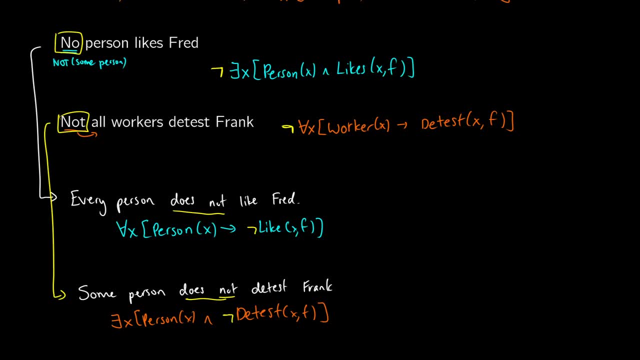 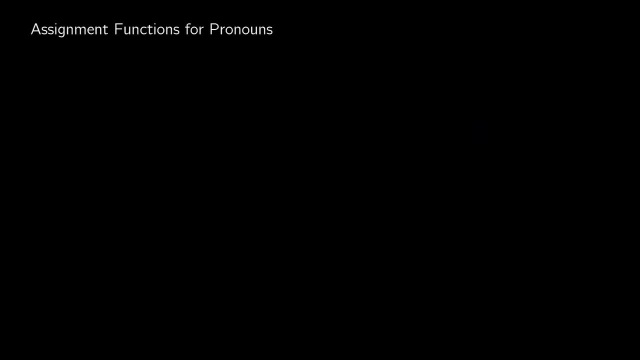 or is going to be inside the formula. Both are completely acceptable. They mean exactly the same things. So for our last bit here I just want to talk about assignment functions for pronouns. We said that if we have a sentence like he sleeps. 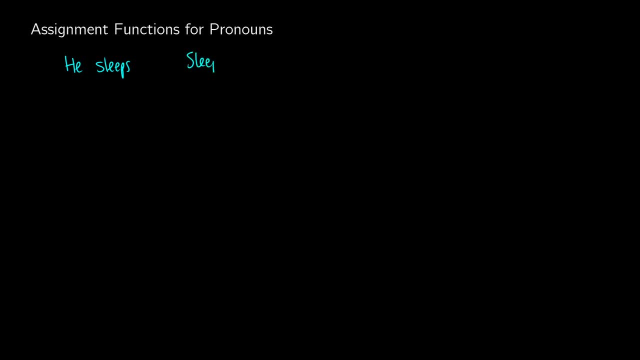 then we would write this as something like sleeps and x. So if we want to know what happens in the real world, we might have what's called an assignment function. So let's call this g, And what it's going to do is it's going to give values. 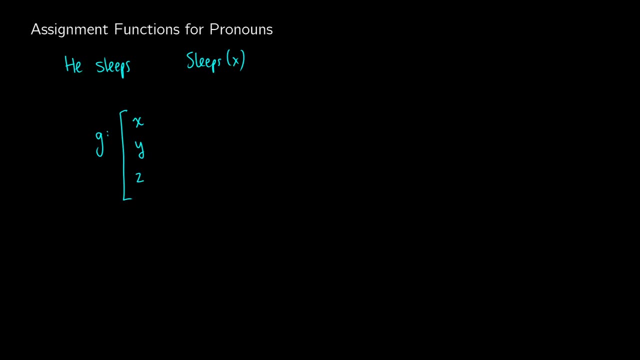 to all of our variables and it's going to assign them to people in our real world. So instead of using x, y and z, we might give them numbers to make them easier. So x1,, x2,, x3, and this goes on to say whatever x we want to go to. 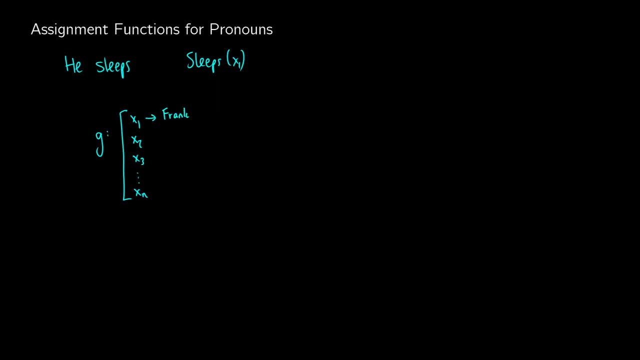 So we might say that x1 is Frank, We might say that x2 is Sue, We might say that x3 is Mary And then x3 and everyone after x3 is also Mary, just to make this a little bit easier to work with. 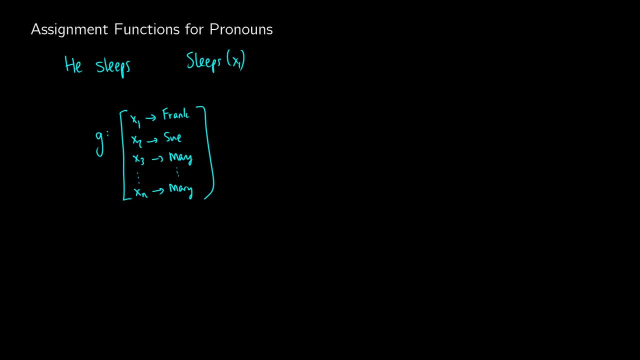 Now, this is something that you decide based on the code, based on the context or discourse. So if you're having a conversation between three people, you would include the people in the conversation and you would include the people outside the conversation. So now we evaluate this function. sleeps x1. 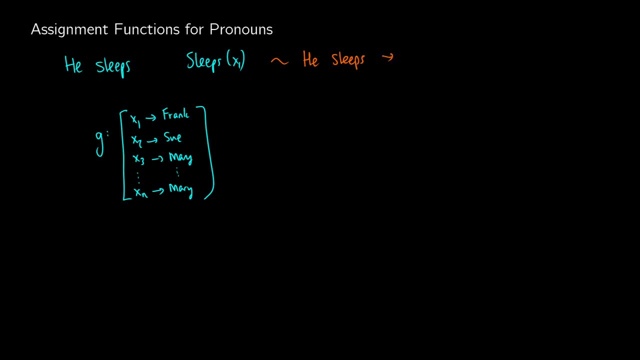 This could still be the sentence he sleeps, but now you know who he is. If we take a look at x1 in our assignment function, we know he sleeps. x1 is pointing to Frank, So this would be Frank sleeps, And we can do this in our predicate logic translation as well.